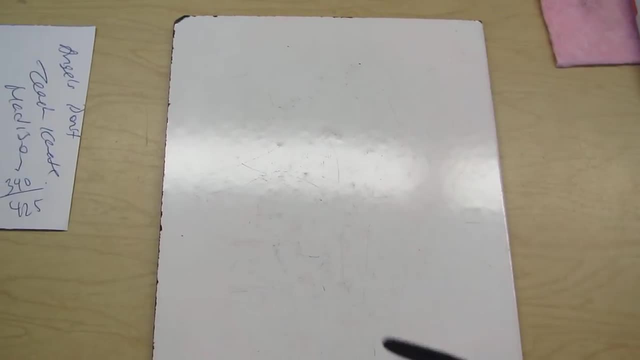 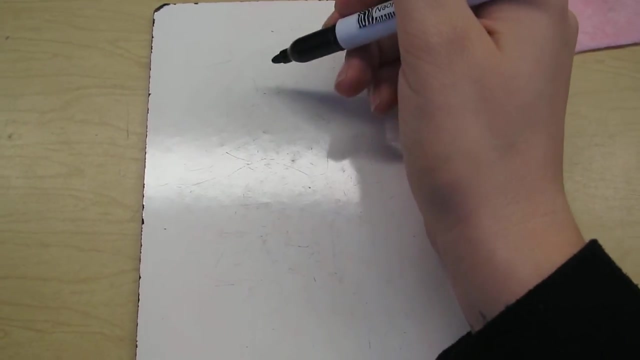 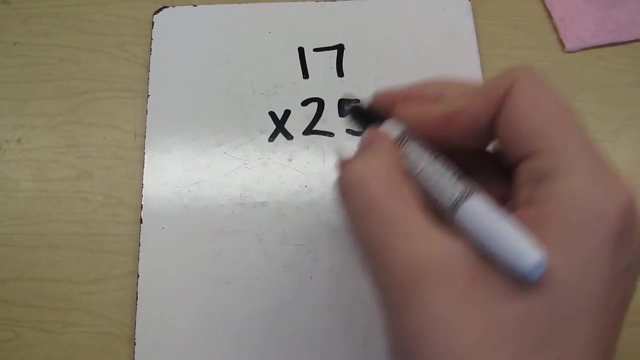 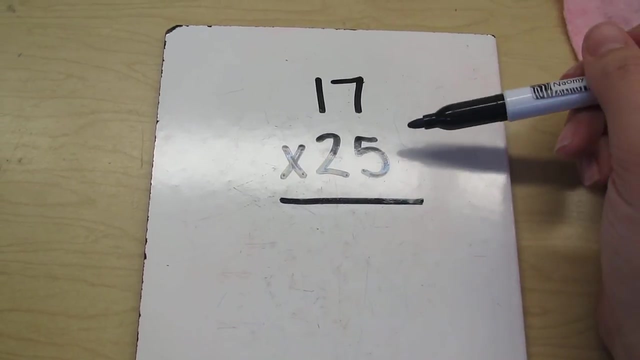 Okay, guys. so, as promised, here is the video on how to multiply two-digit numbers. So the example that we're going to try with is 17 times 25.. Okay, so, like we talked about in class here, what we're going to start with is the number in our ones place. 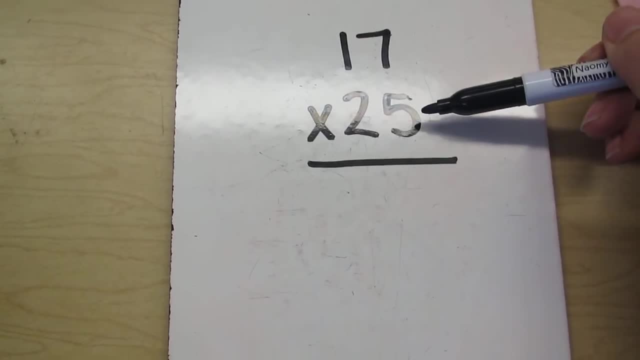 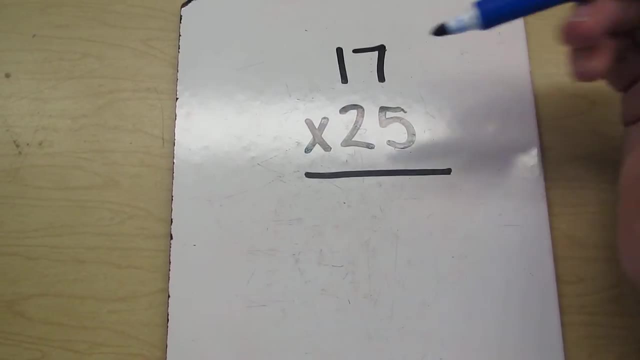 So the number in our ones place on the bottom here is the 5 in 25.. So we're going to start by multiplying those numbers first And I'm going to change colors so you can see what I'm doing properly And you don't have to change colors if you don't want to. but maybe to start off, 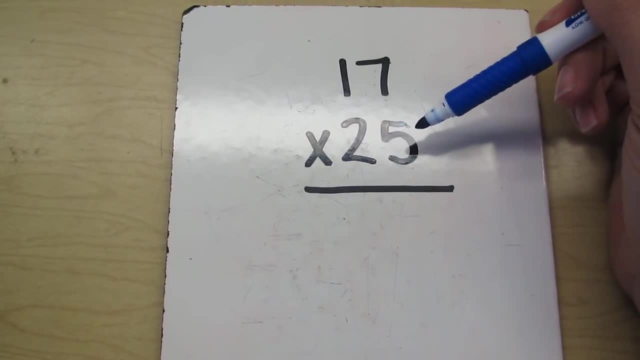 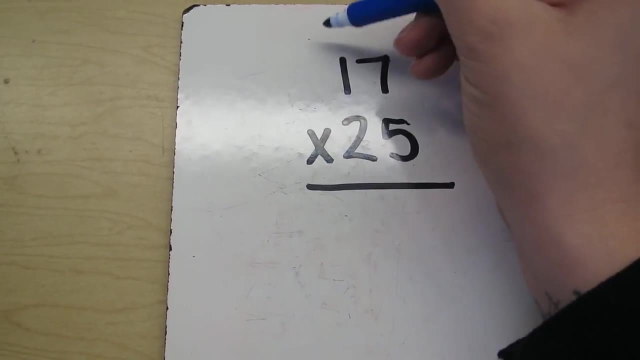 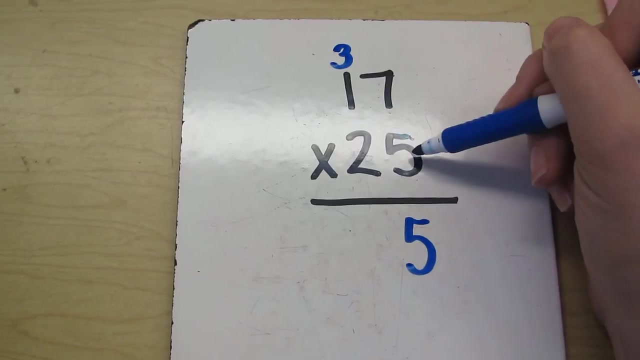 I would recommend it just to see what steps you're following. So first we're going to do 5 times 7.. 5 times 7 is 35, so you put 3 up here And a 5 down here. Okay, then we're still working with our ones. 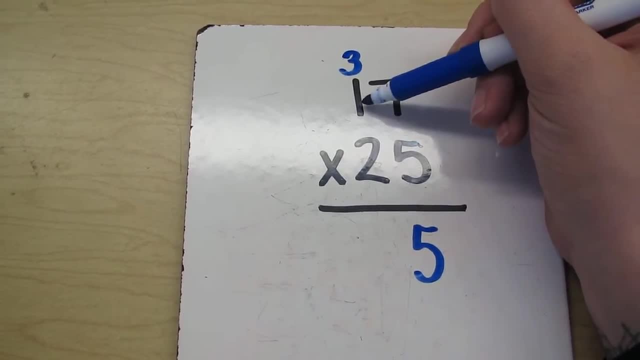 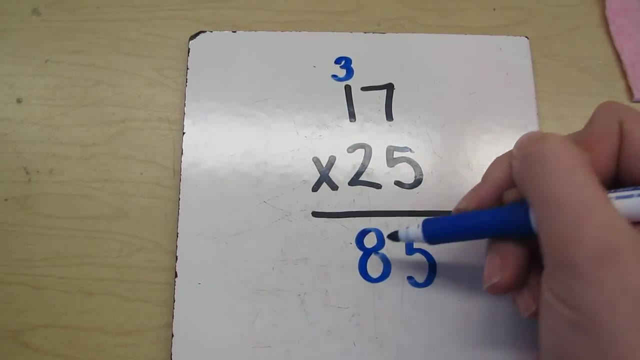 So we're doing 5 times 1,, which is 5,, plus 3,, which is 8.. So 5 times 1, 5, plus 3, 8.. So now this means that I'm finished working with my ones. 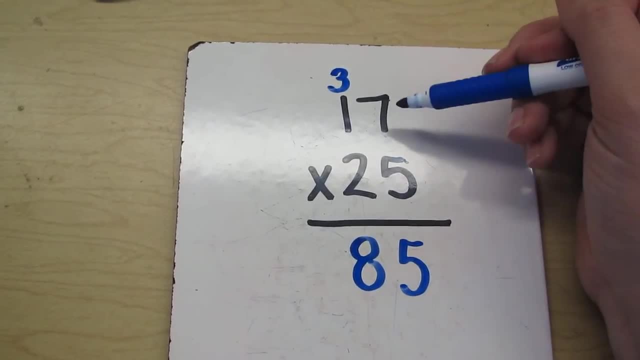 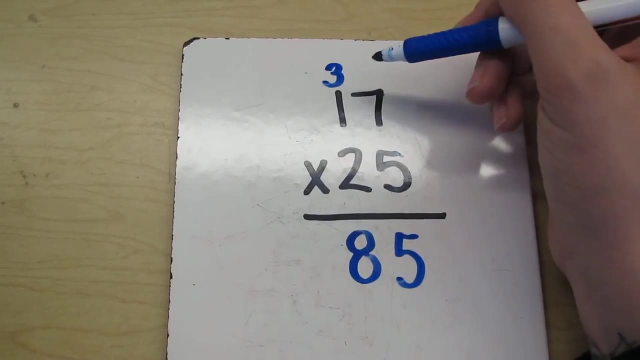 If you remember the base 10 blocks, technically what we just did was 5 times 17 gave us 85. So we're finished working with it. so there's three steps when we're finished. First, we cross off whatever we did on top, because we don't want to get confused. 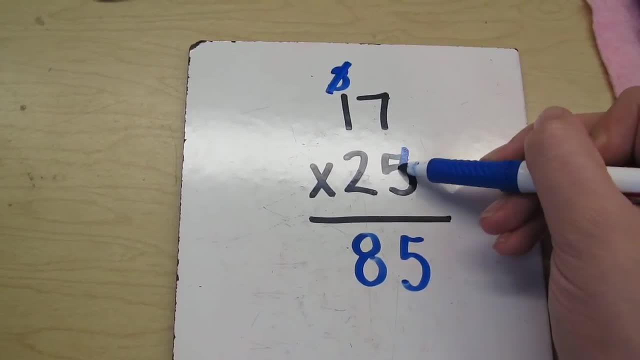 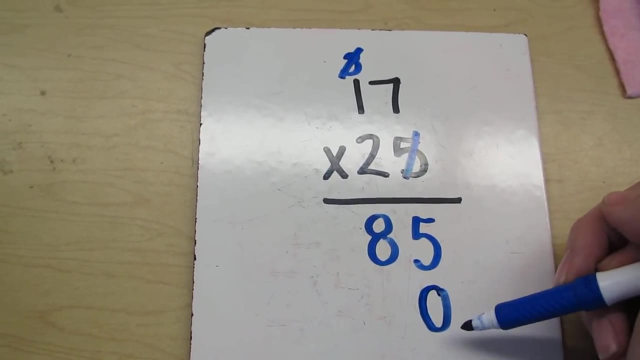 We don't need it anymore. Then we cross off our ones place. We're also finished with that, And because we're finished, we have to add our 0 down here, because it means we're working with the tens place now. So let me change colors again to show us working with the tens place. 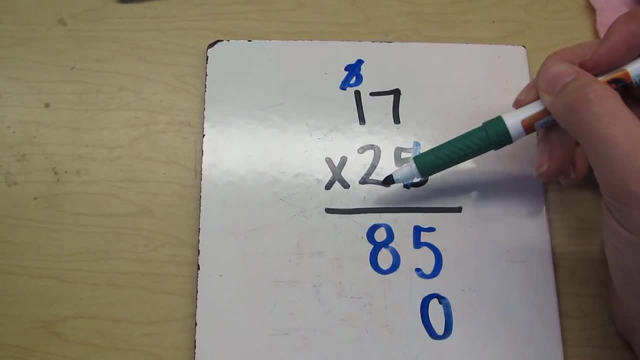 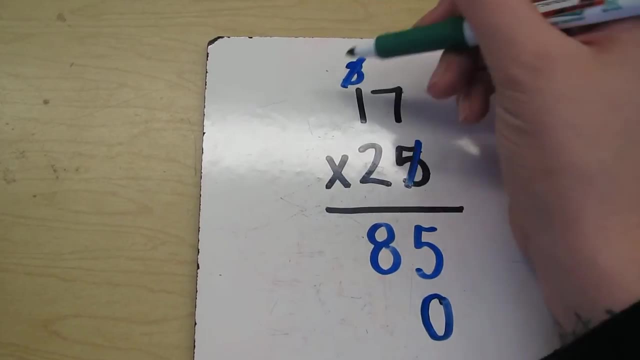 So now at the bottom here our tens place is the 2.. So we're going to start multiplying with our 2.. So first we have 2 times 7,, which is 14.. And again the 1 goes up here. 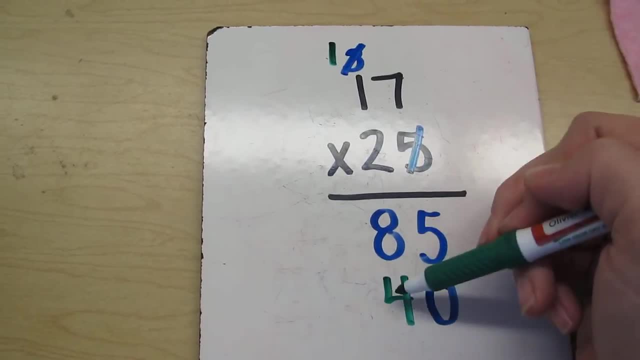 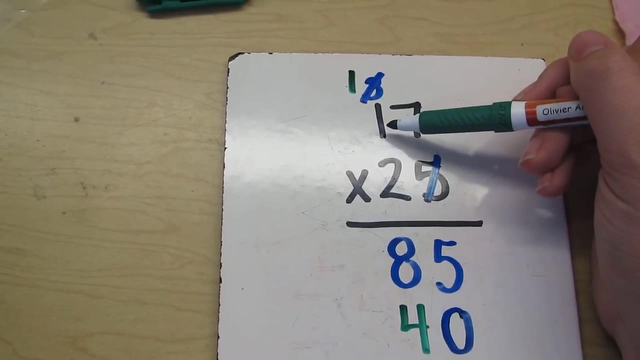 1 and 4 for 14.. 1 and 4.. And then we're going to go to our 2 tens place. We have 2 there and 1 there, So 2 times 1 is 2, plus 1 is 3..